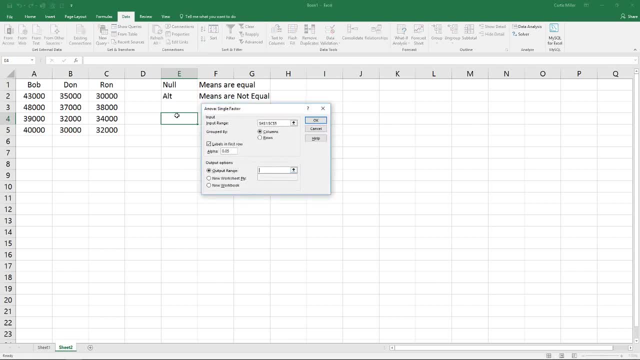 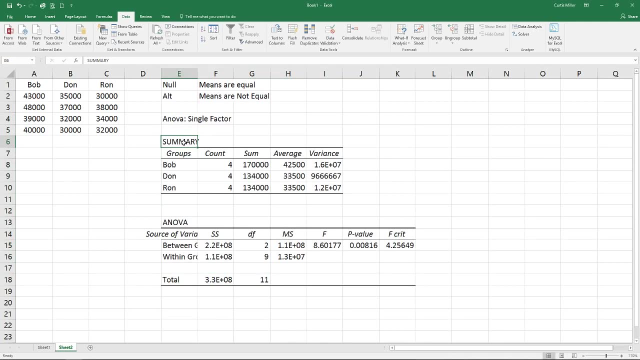 So our output range I will select right here below my hypotheses. We will let that come out. So we notice here our ANOVA single factor. We start with our summary data. So for each one of our doctors, Bob, Don and Ron, we had four records. 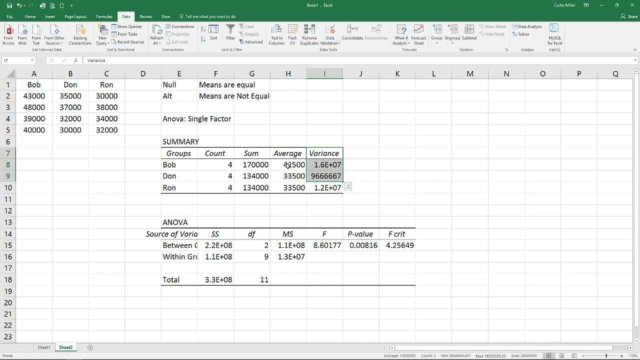 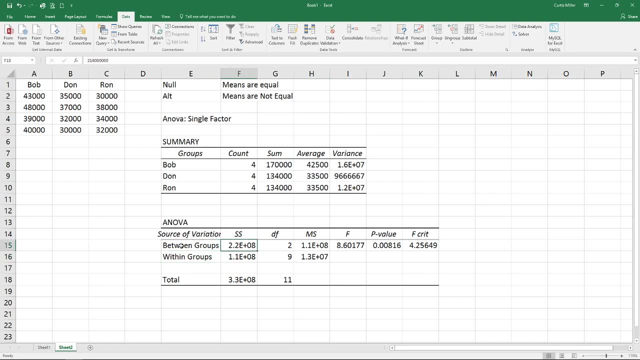 We had their sum, their average and their variance. Now, if we look down here at our ANOVA table, where we find the data we are most interested in, We are going to concentrate here in our between group section, where we have data for some of the squares of the errors. 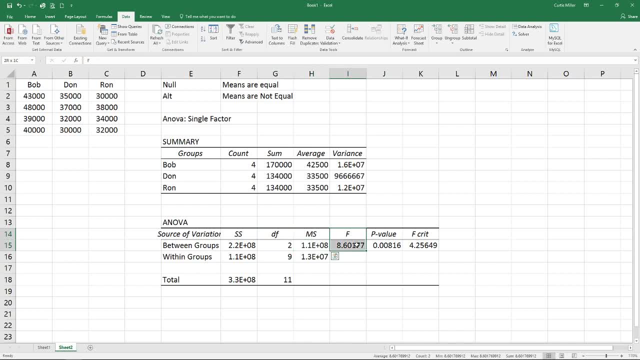 The degrees of freedom, the mean squared error. And then we have our F value And our F critical. Now for these. we are going to compare these similar to what we did for our two group hypothesis test, In that if the absolute value of our F is greater than our F critical, which is our rejection point- 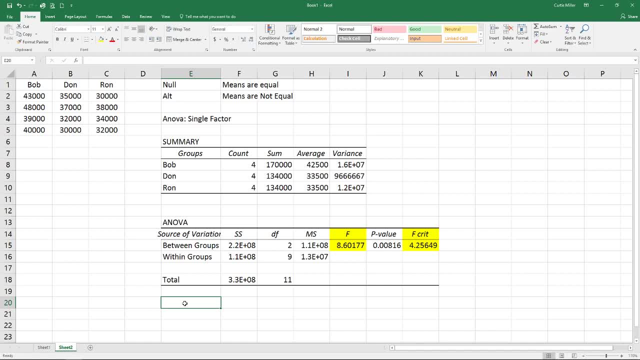 Then we will assume our null hypothesis is incorrect and we will reject that, Which is the case here. So because our F, our absolute value of F, is greater than F critical, We reject our null. So that means we will assume our means are not equal. 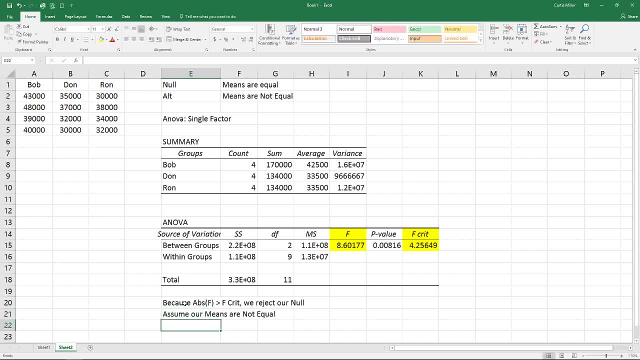 Now, unfortunately, at this point, if we wanted to determine which means were different than the others, We would need to go back to our two group hypothesis testing And perform tests On Bob versus Don, Don versus Ron And Bob versus Ron In order to figure out which ones are different. 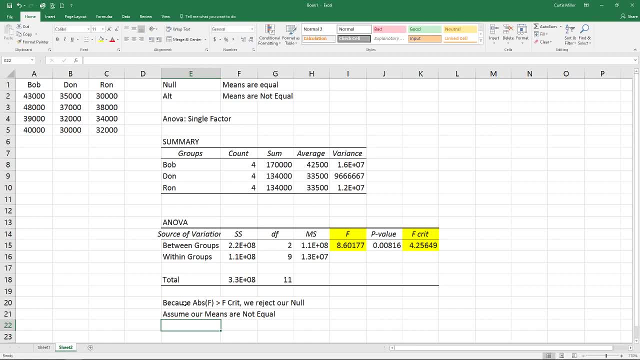 However, had we come to the opposite conclusion, Where we accepted our null hypothesis, We could complete our test and be done. That's really all there is to ANOVA testing- The very simple basics of how to perform the test. Hopefully you found this video useful. And thank you for watching.